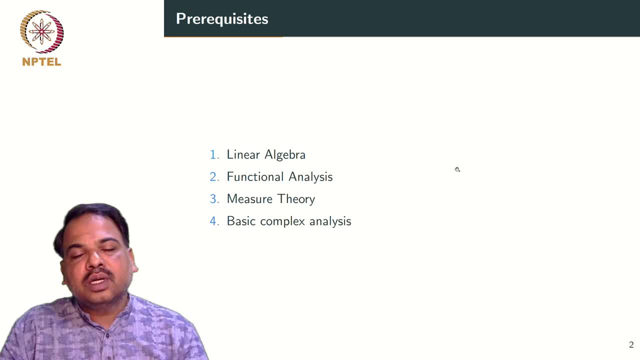 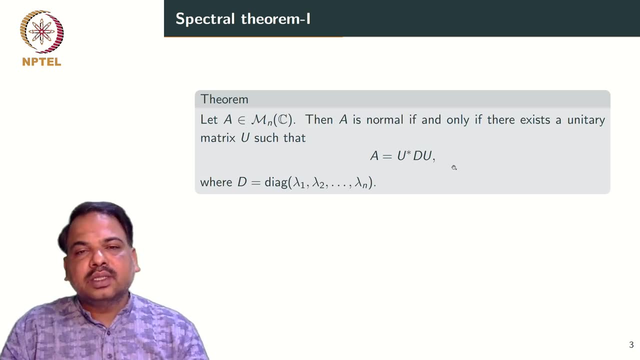 the analyticity of functions, Cauchy integral formula and the Lewis theorem. Let me quickly recall two important results from basic linear algebra. If A is a n by n complex matrix, then A is normal. if, and only if, there exists a unitary matrix U such that: 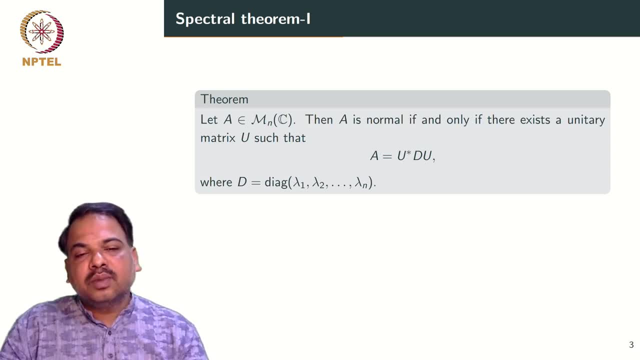 A equal to U star du, where d is the diagonal matrix with diagonal entries: lambda 1,, lambda 2, so on lambda n. The values of d are exactly eigenvalues of A And in fact unitary equivalence preserves the trace, the determinant, invertibility and many more important properties. 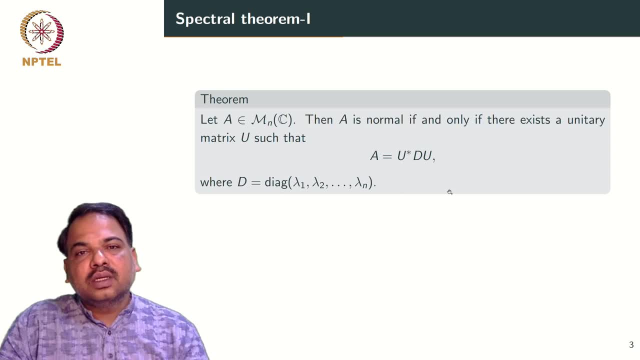 So by expressing A in this way, we are going to get information about A from the matrix d. So since d is a linear, d is a matrix n by n matrix, it can be viewed as a linear transformation from C? n to C n. 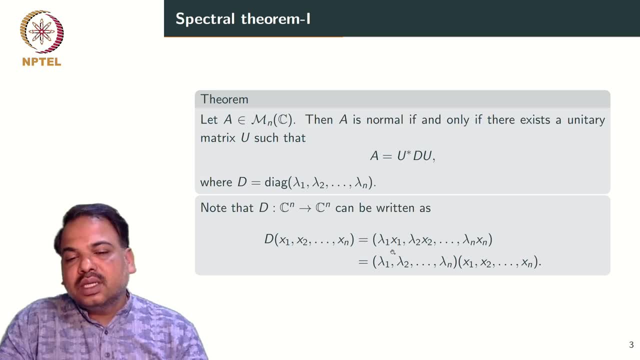 A can be written as d of x1, x2, so on, xn equal to lambda1, x1, lambda2, x2, so on lambda n, xn, And this can be written as pointwise product of these two vectors, lambda1, lambda2,. 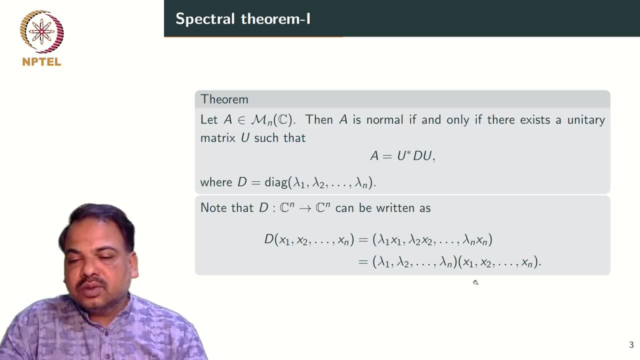 so on. lambda n multiplied by x1, x2, so on xn. That means the diagonal matrix d or diagonal operator d. we can view it as a multiplication operator with a fixed vector: lambda1,, lambda2, so on xn. 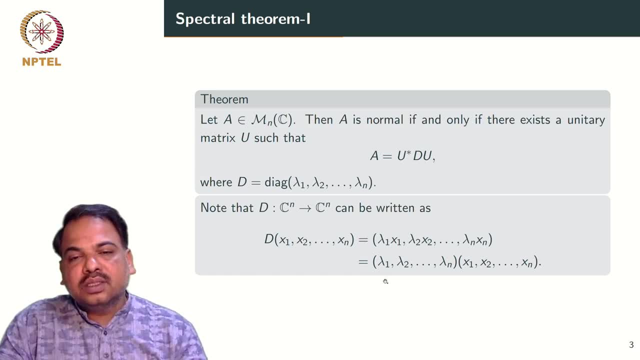 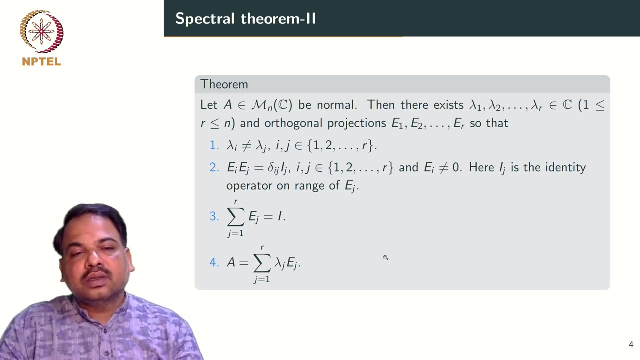 so on. lambda n. This representation of D is going to be very useful when we want to extend this result to the infinite dimensional setting. Let us recall one more important result from linear algebra: If A is a n by n normal matrix with complex entries, then there exist complex. 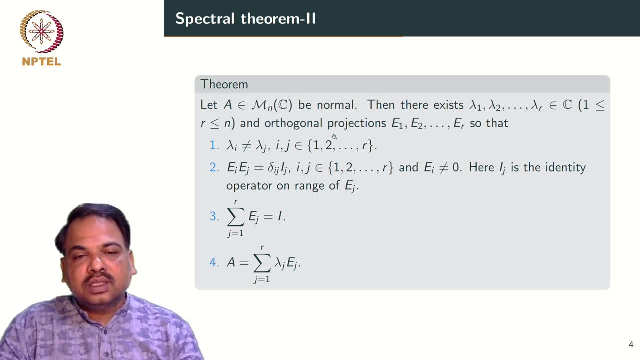 numbers, lambda 1, lambda 2, so on, lambda r, which are distinct and orthogonal projections, E1, E2, so on er such that they are mutually orthogonal in the sense that range of Ei is orthogonal to range of Ej, for i not equal to j, and each of them is non-zero. and the third condition says: 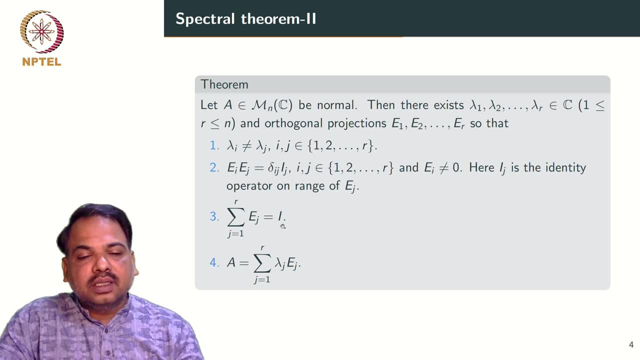 that summation j equal to 1 to r, Ej is identity. So this can be expressed as follows: c power n can be splitted as orthogonal direct sum of eigen spaces of a, and the fourth condition says that Ej is a, n by n. normal matrix with complex entries. then there exist complex numbers, lambda n. 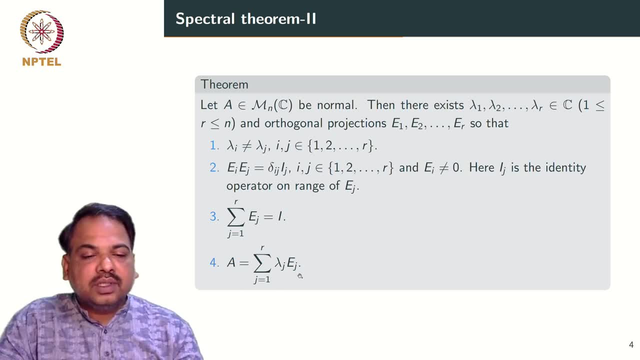 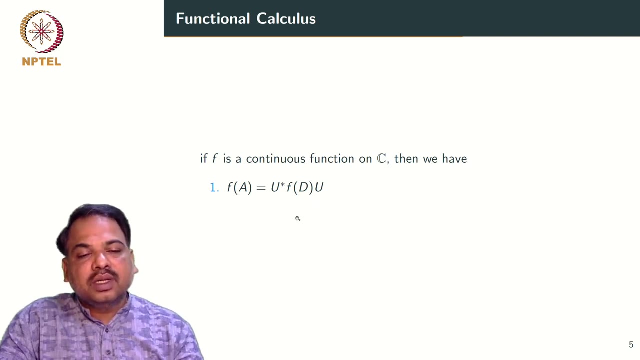 summation j equal to 1 to r, lambda, j, e, j. that means we are writing a as linear combinations of orthogonal projections onto the eigen space. and further, if f is a continuous function on c, then we can say that f of a can be written as: 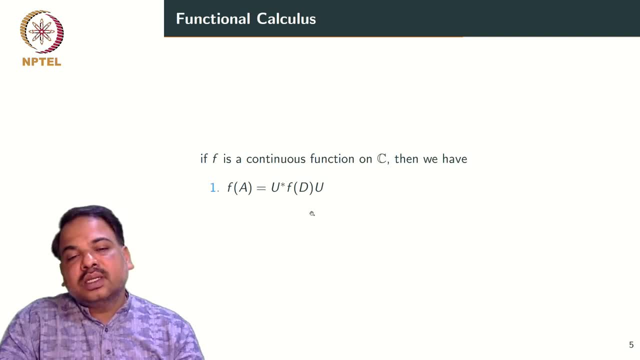 u star f of d? u, where d is a diagonal matrix with diagonal entries: lambda 1, lambda 2, so on lambda n. in this case it is easy to look, easy to find out: f of d, which is a diagonal matrix with diagonal entries: f of lambda 1, f of lambda 2, so on f of lambda n. so in the second case, f of a can be. 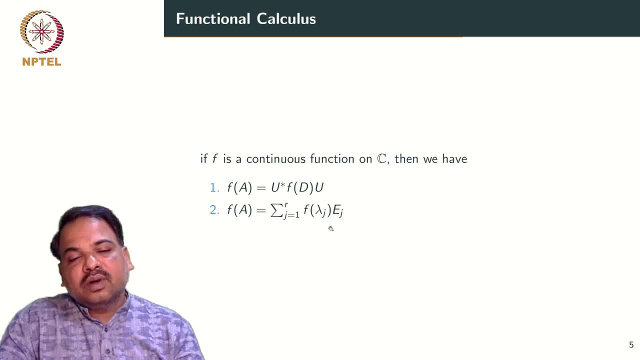 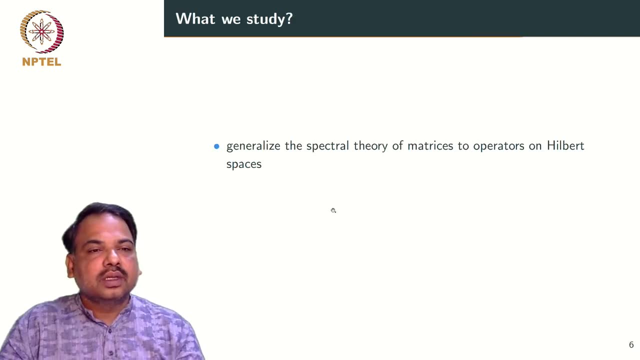 written as follows: summation j equal to 1 to r f of lambda, j e, j. so in this course, what exactly we are going to study? our aim is to prove all the earlier results. so in this course, what exactly we are going to study? our aim is to prove all the earlier results. 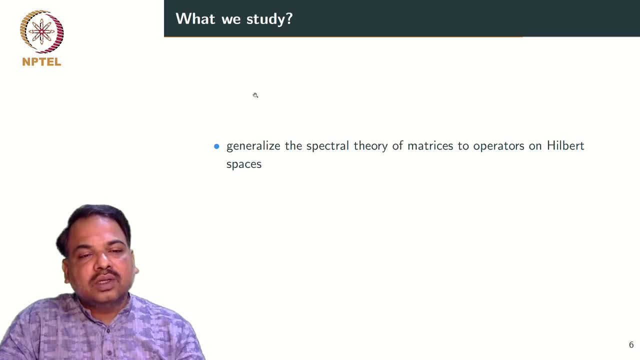 to the infinite dimensional setting. in other words, we want to generalize the spectral theory of matrices or finite dimensional operators to operators on infinite dimensional liberal spaces. so in this case we have to actually replace the set of all eigenvalues with an appropriate set that we call as a spectrum of an operator, when we restrict the operator to finite dimensional space. 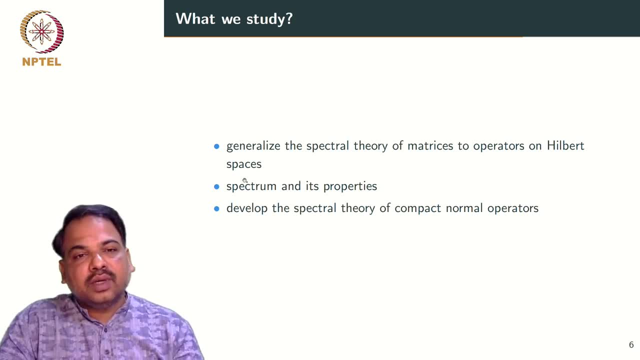 the spectrum exactly coincide with the set of all eigenvalues. it is possible to find examples on infinite dimensionalunivers spaces with out eigenvalues. in that case, spectrum is a more generalization of set of all eigenvalues and in this course we are going to look at different kinds of operators and